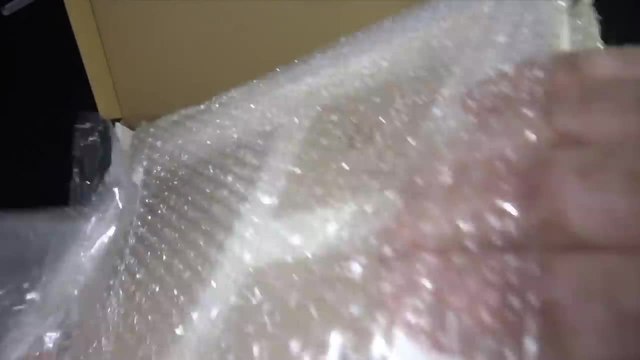 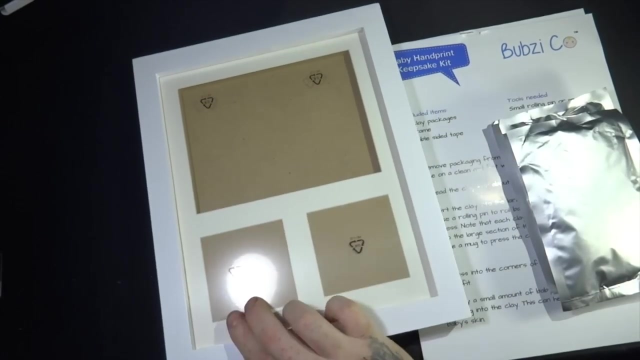 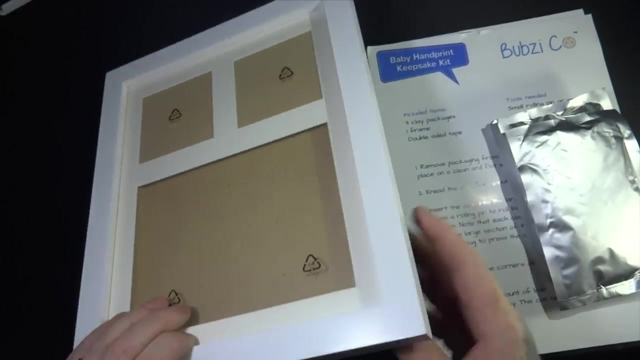 So you've got three packs of that And then we've got the frame itself. So let's take this out, Okay, so I'm going to be using this and film it so you can see exactly how we get on with it. So the frame unclips from the back. It's a nice frame. It's solid wood. 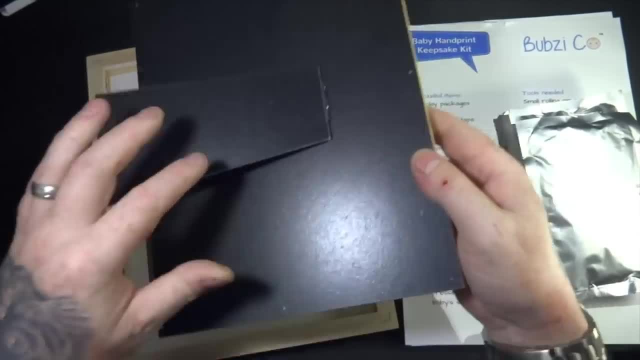 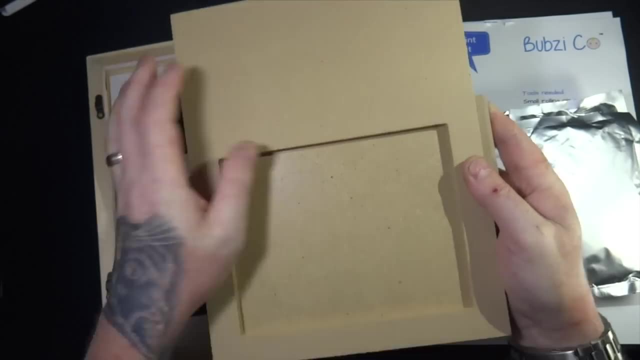 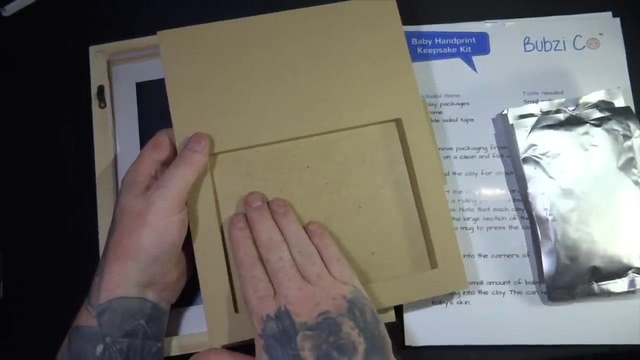 So it's nice, nicely made, Cool, that's proper thick, So the whole thing is in one there. It's made out of MDF, So you obviously need all this clay together. Fill in this gap here, And this is where you put the hand and the foot. 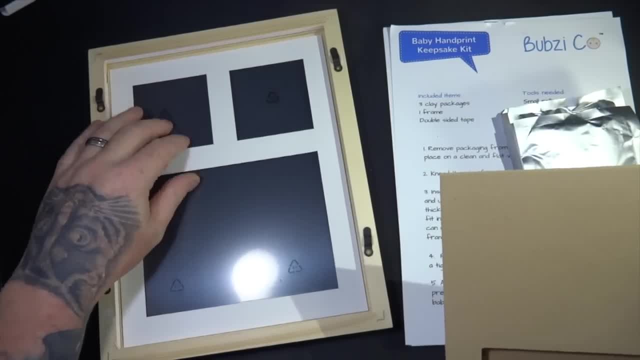 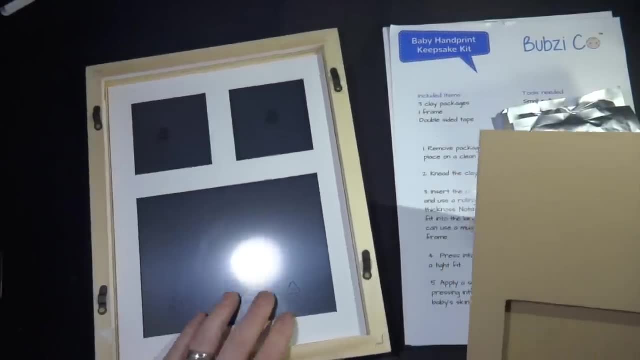 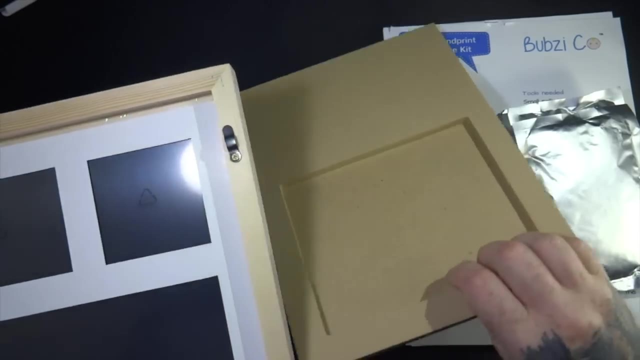 And then, obviously, you've got the cut outs for the hand and foot And you can have a picture in each side, And the glass has got a sticky backing on it just to stop it getting scratched. I'm going to leave that on for now. 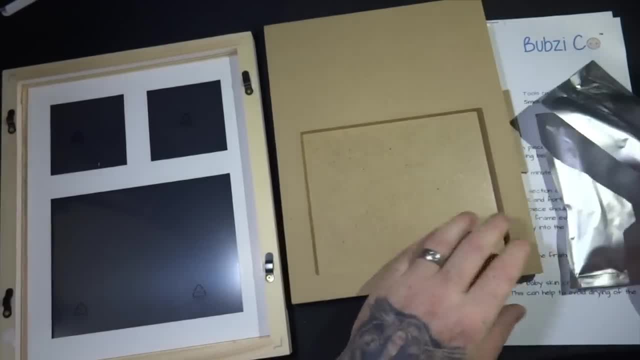 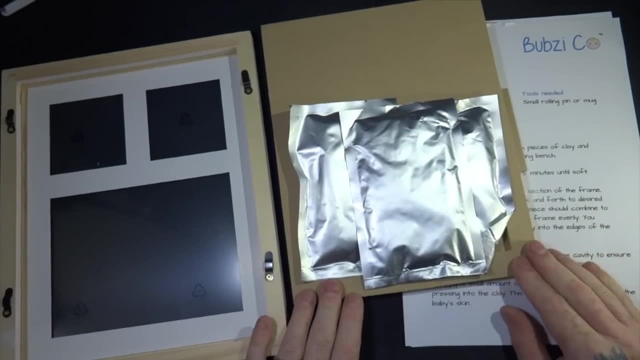 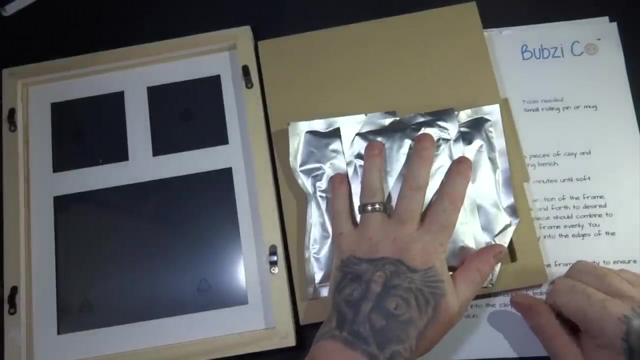 But I'll set all this up and show you how it works. So the next thing you'll see will be us manipulating my grandchild into putting his hand and foot into this. I hope this all works out Right. okay, so I've got the three packets. 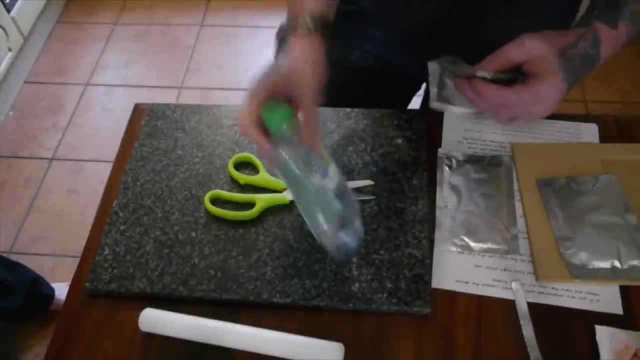 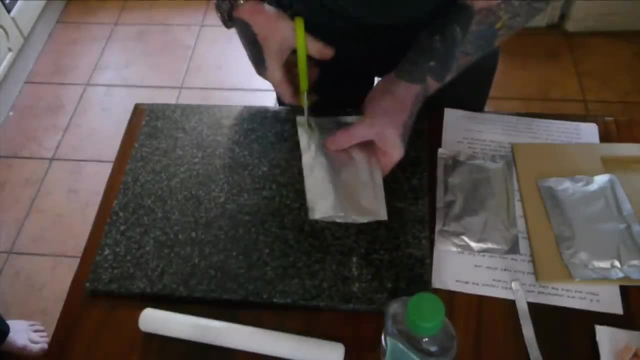 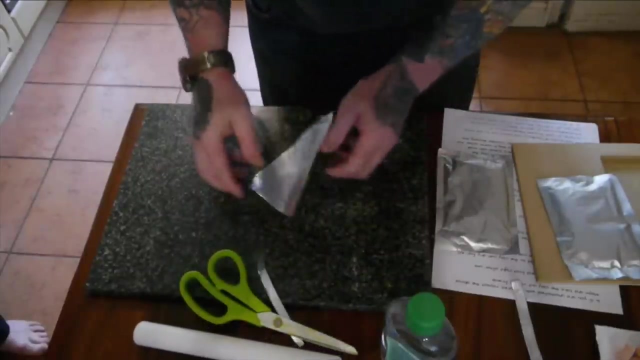 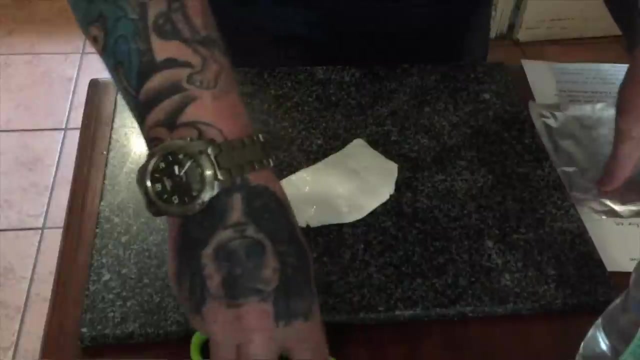 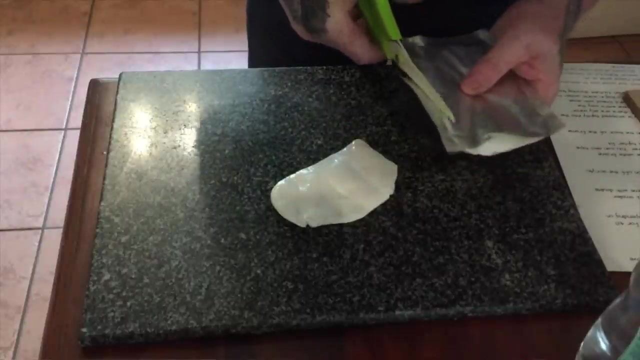 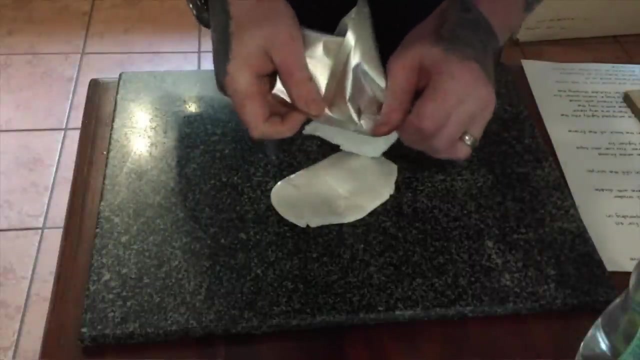 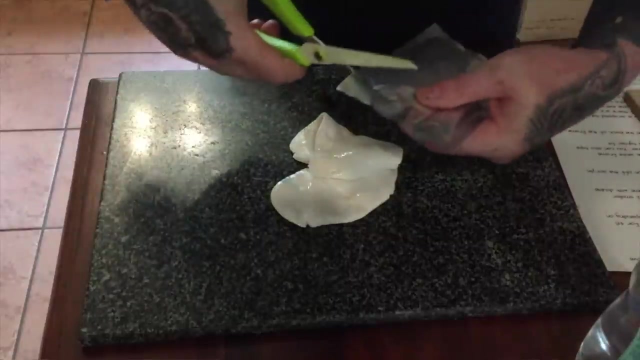 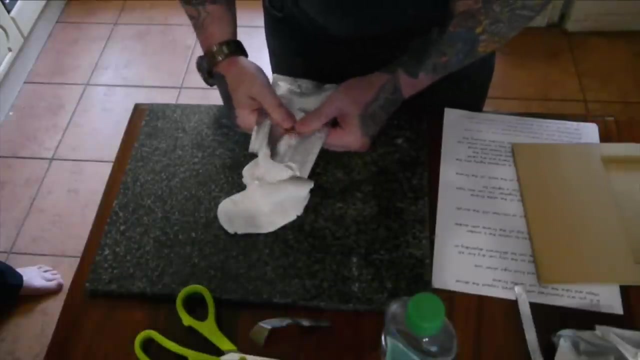 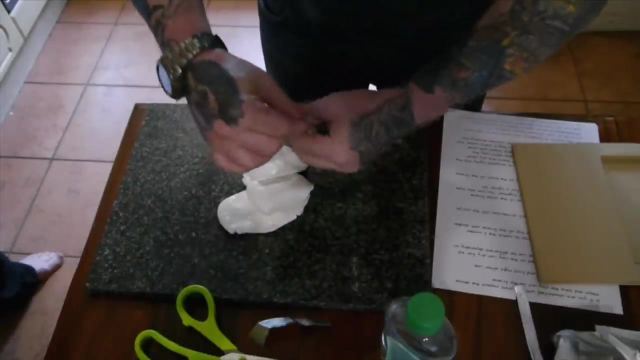 Also got some Johnsons Baby Oil- Going to empty the packets out And we're going to be using these for the first time It recommends. on the third one, you save some in case you need to fill any cracks in after. I'm just going to keep that sealed up because we don't need any repairs. 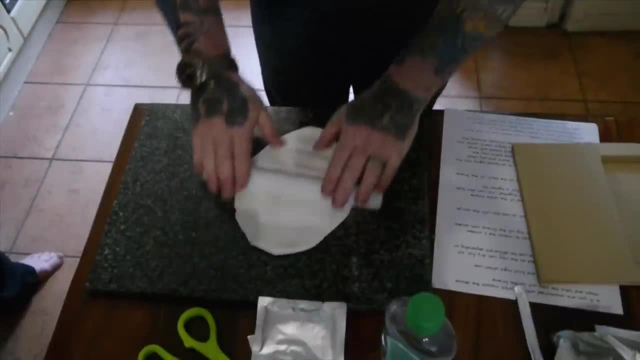 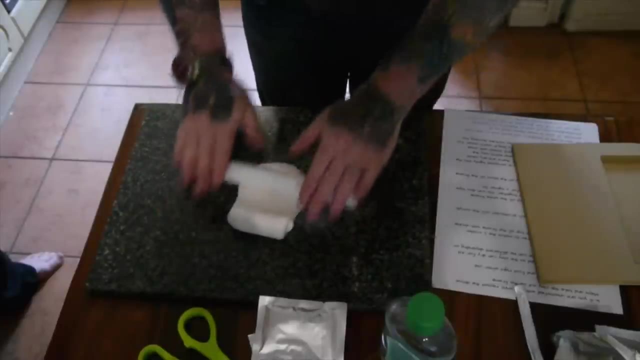 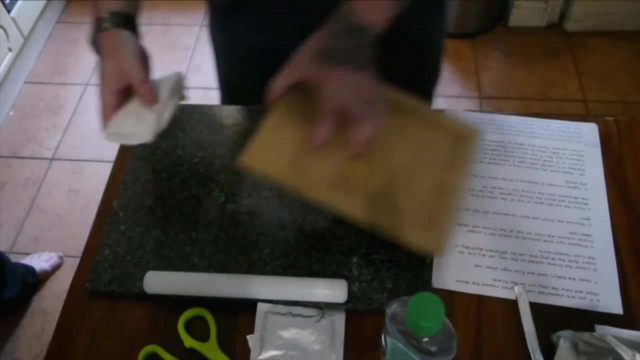 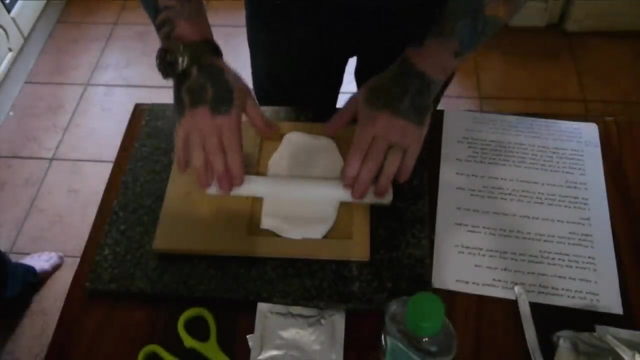 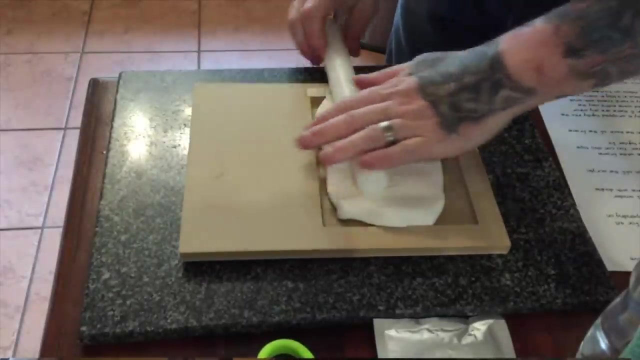 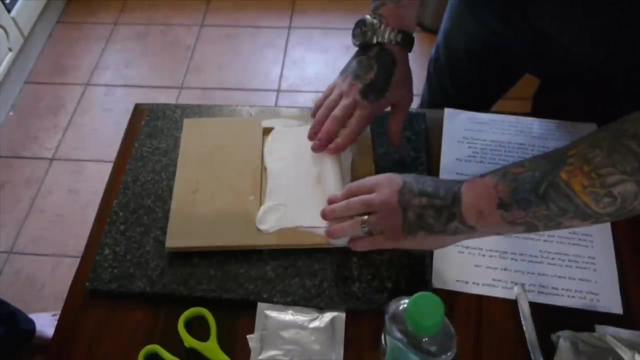 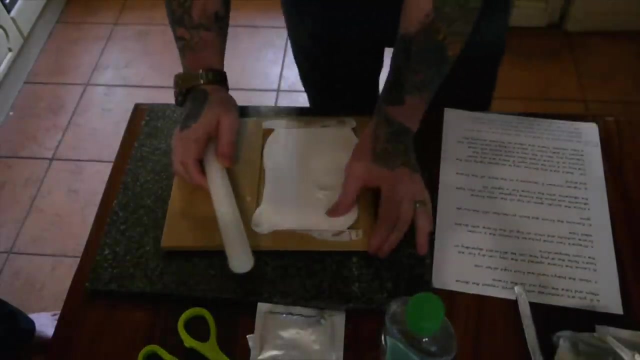 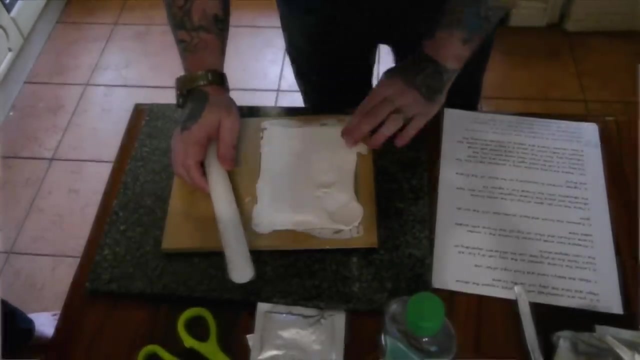 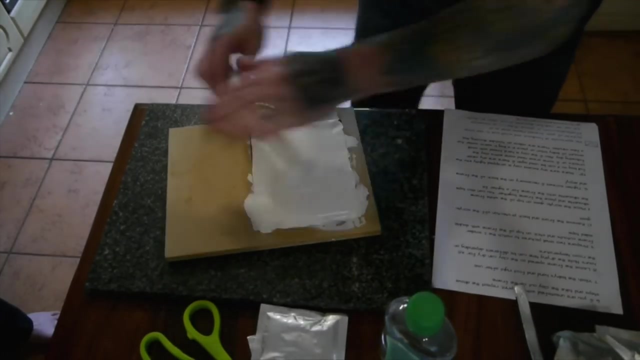 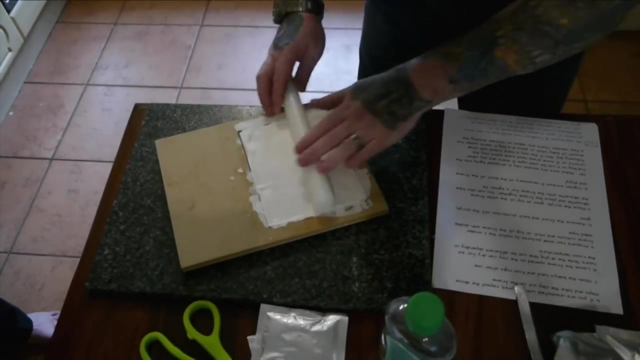 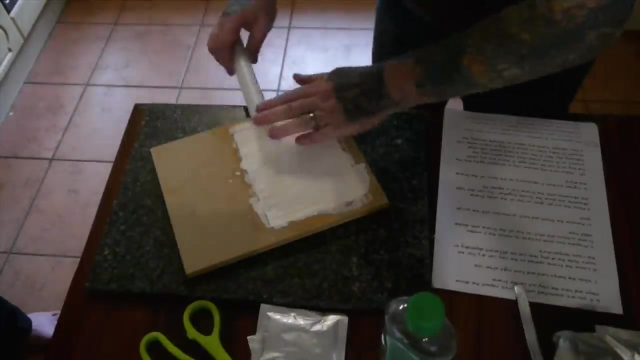 Just think we've got pastry. give it a good roll now stick it in. make sure you get all the way through. It's going all the way through the corners, But it's going to be pretty quick. You don't want to pull it out. 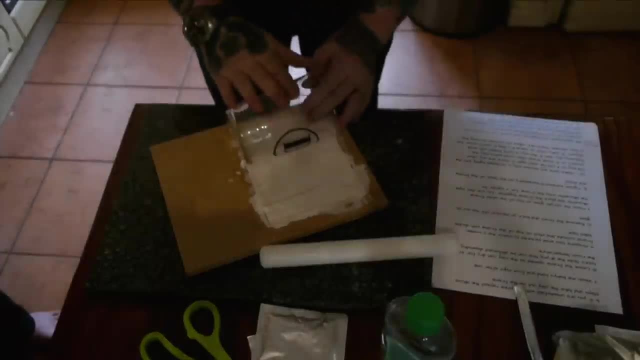 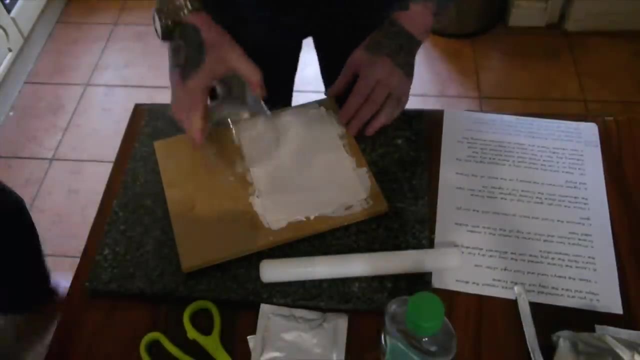 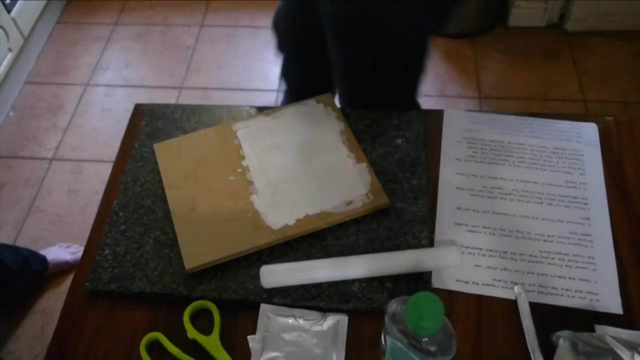 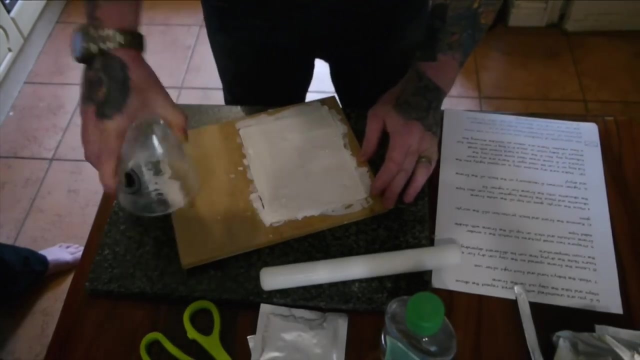 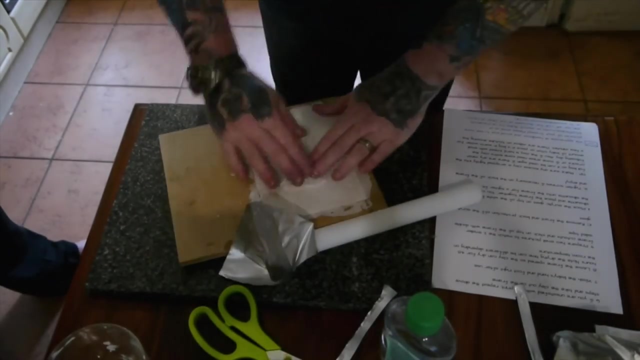 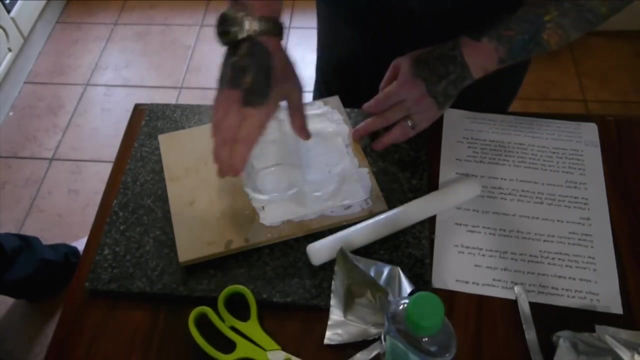 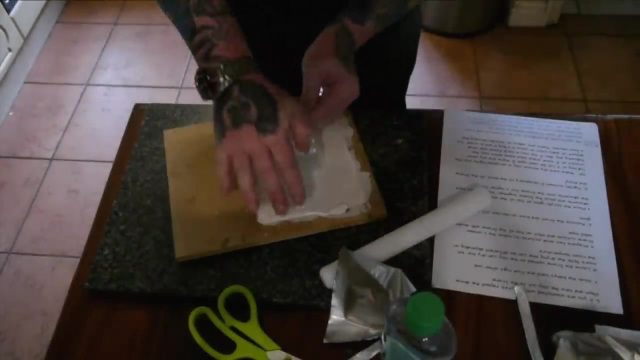 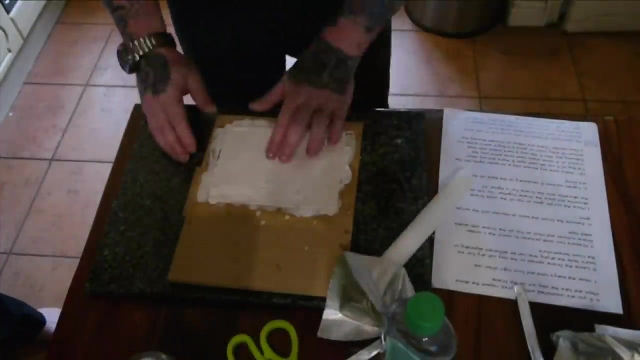 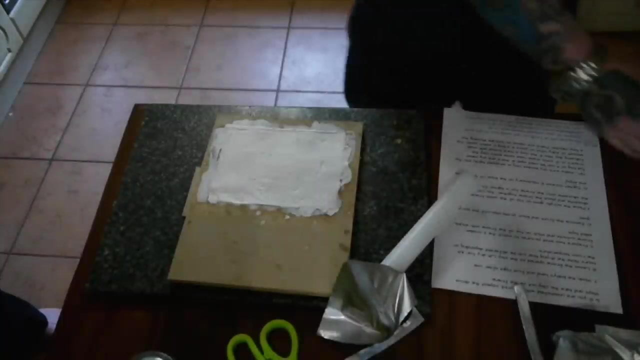 You don't want to pull it out. There we go One foot, the foot there and the hand there. Oh yeah, of course it is. What are you going to do? Do opposite hands? I'm going to do right foot. I know. this is why I'm doing this now. 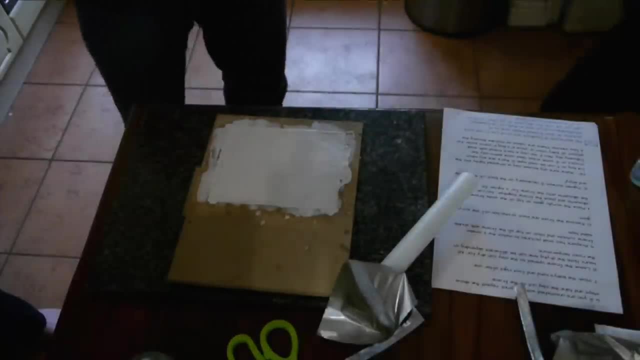 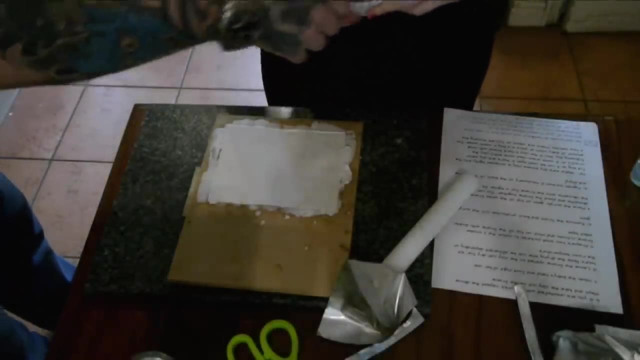 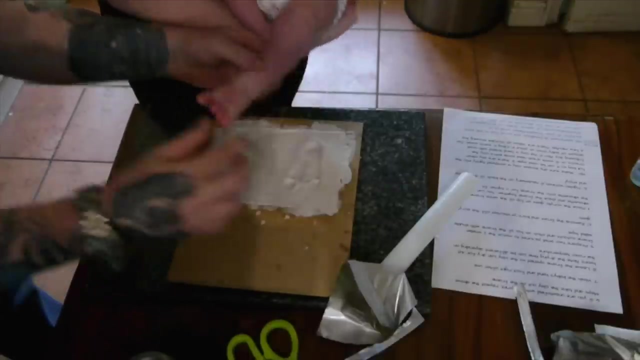 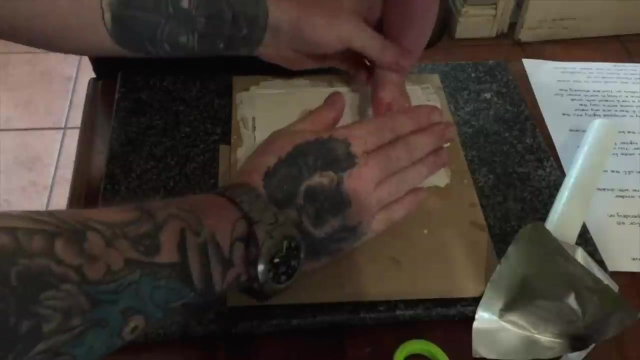 Smell the oil. Ok, so we'll do the foot first And turn him around more. so it's more level now. Come on, that's it. Put his foot down. Don't forget his toes. Ok, He's wiggling his toes. Ok, that's good. 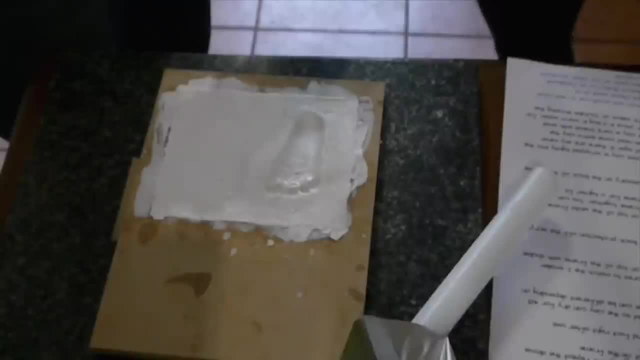 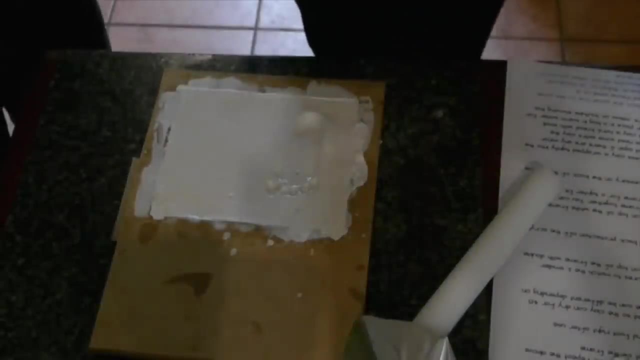 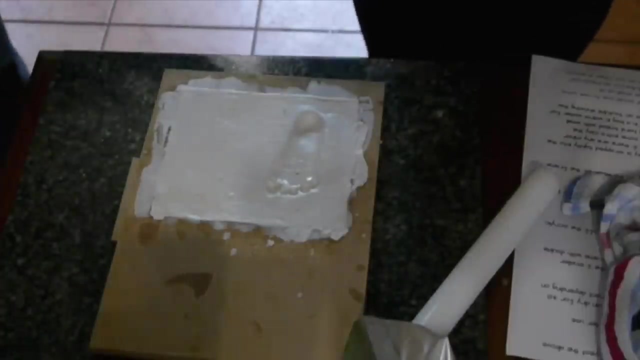 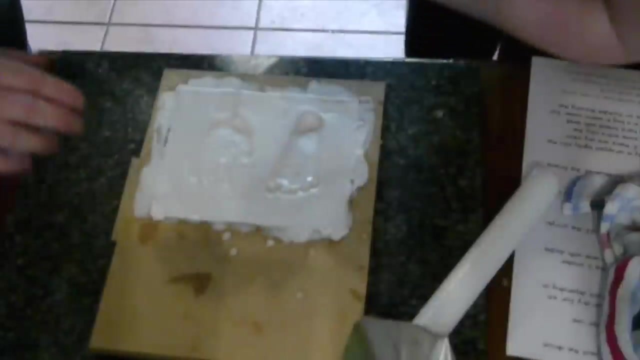 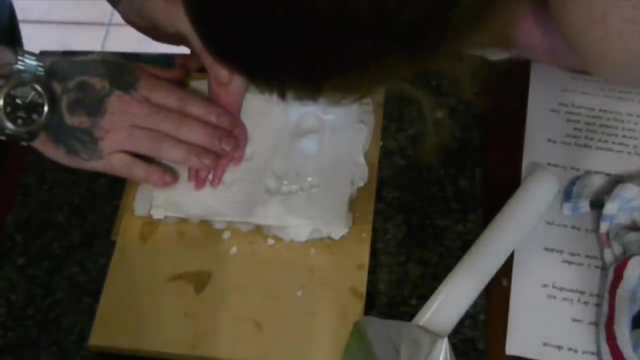 Now his hands Right hand. This is going to be a tough one. Yeah, it might be. It might be pants. Right, you're going to get him down there Right hand up, Not quite. you do it again. Hi, buddy, Right, he's done two hands now. 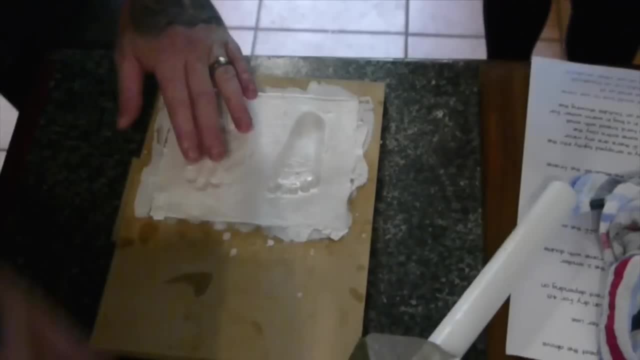 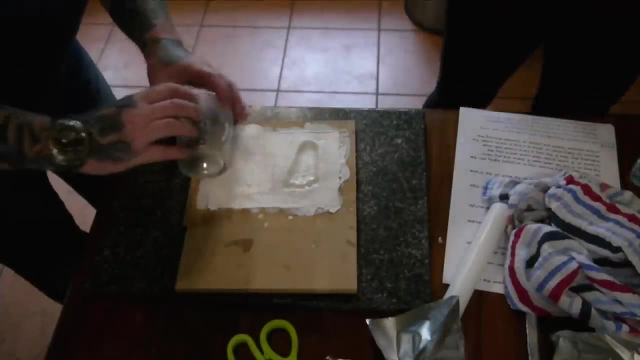 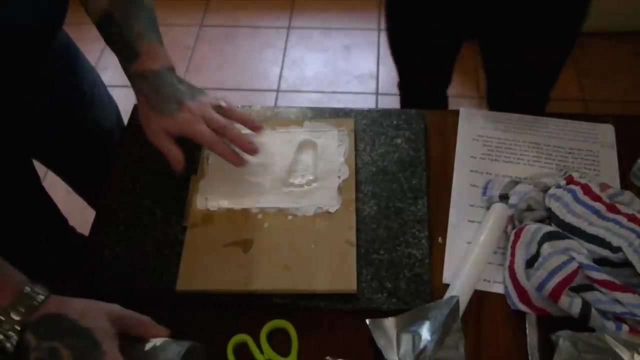 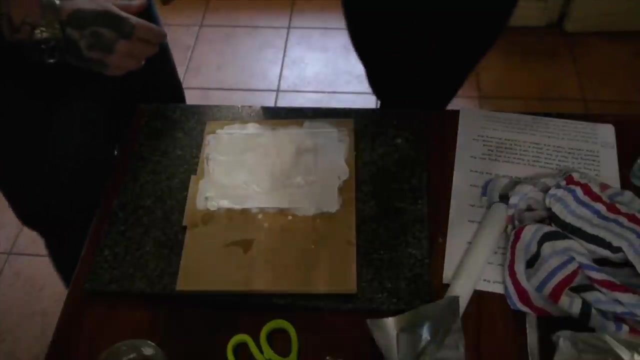 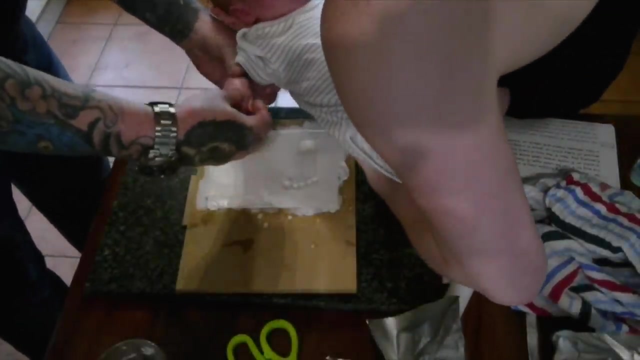 He's all over the flat line. Sorry. sorry, I just don't want to push his hand too hard, Unless you hold him and I push it, Because you can paint it anyway to make the hand stand out. Ah yeah, What are you doing? I know. 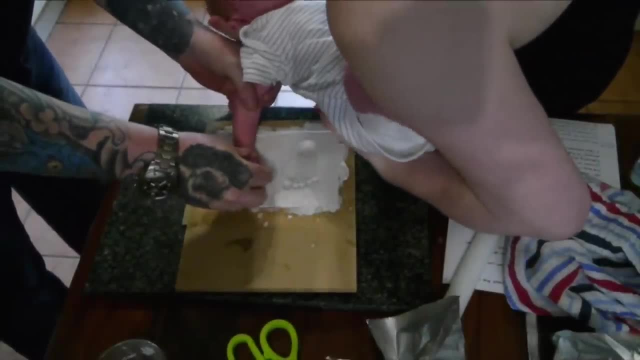 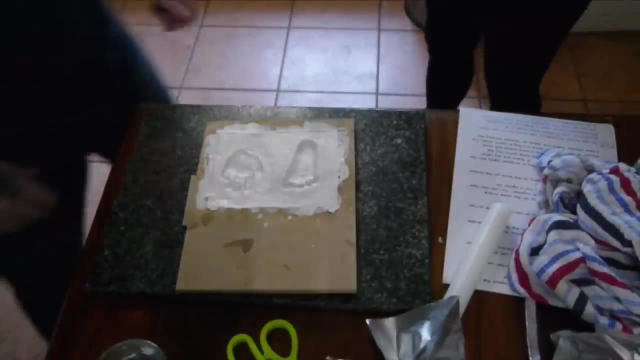 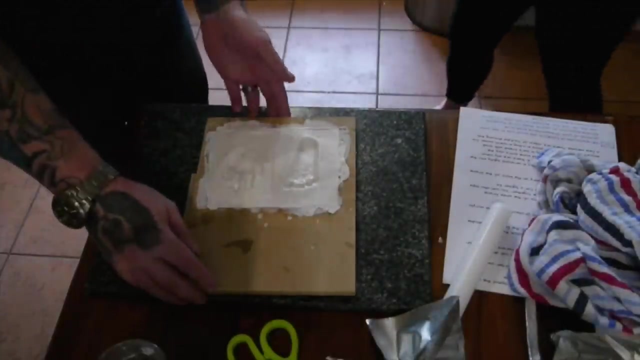 He won't be able to relax his hands. Oh baby, I know That's fine. There we go. Shall I leave that to dry now. One, two, three, four, five. Yeah, His foot's really good. The foot's really well different, The hand was a bit harder. 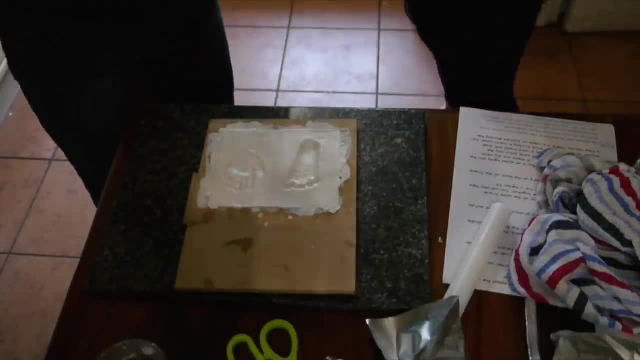 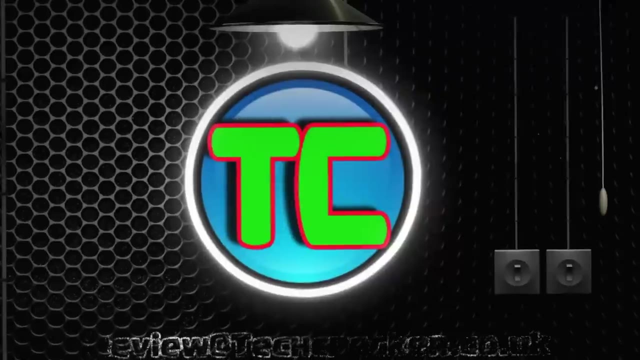 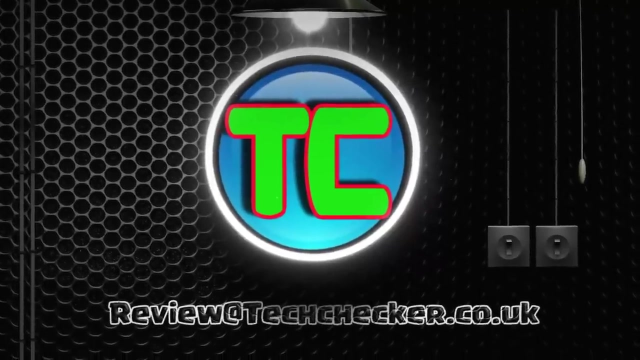 But you can still see it. So yeah, there we go. Okay, let's do it again. One, two, three, four, five. See, that's a really good one. I'm sorry. Okay, I'm done. It didn't take long, We're good.